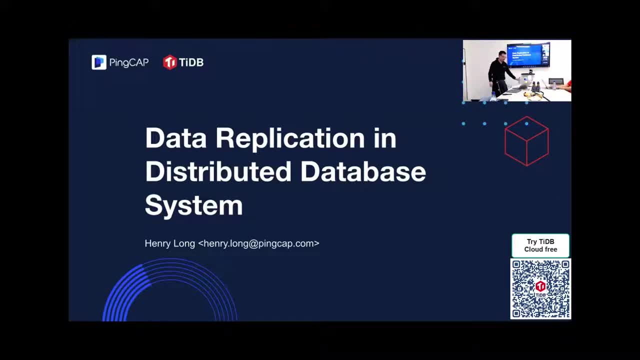 Hi everyone. I'm Henry. Today's topic is data replication in distributed database system. It's not natural if you don't know much about distributed database system or data replication. Hopefully this topic can make you understand deeply the scenarios of the presentation and how to implement it in database system. I'm Henry Long. I joined Pink App. 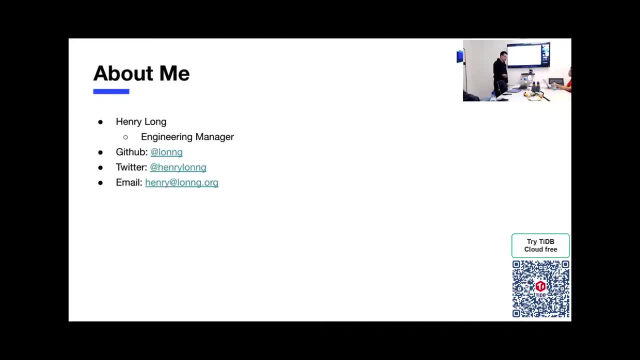 for the past years I contributed a lot of components in TidyView, For example, the data ingestion, the data replication back cover store and TidyView Cloud deployment tools. Now I run the data platform team focused on the data flow system. 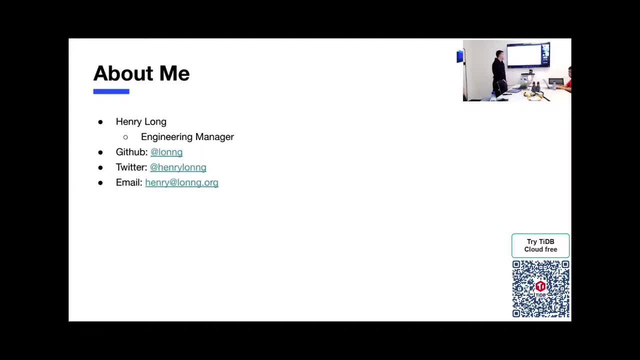 for TidyView. This is my GitHub. Before I joined Pink App, I launched an open source project. I love open source, so I joined Pink App to build an open source database system. This is my Twitter and my email. Any questions about open source and database. 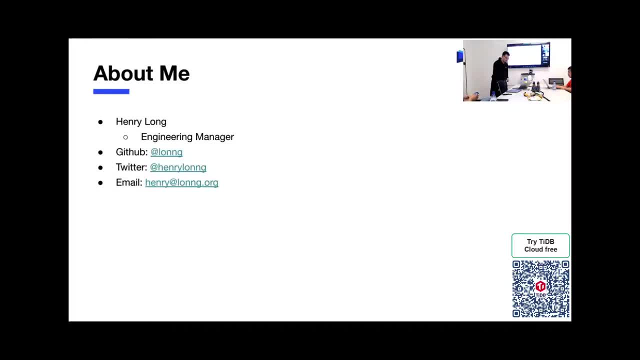 welcome to contact me for a further discussion. For today's topic we are speaking about data replication in distributed database system. I will introduce the concepts and the scenarios of data replication to make sure we are on the same page. Then I will introduce the design and 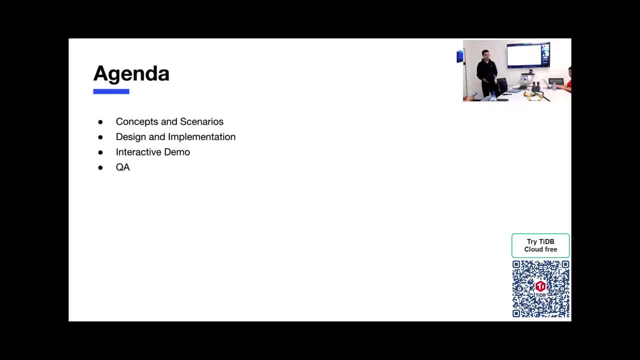 the implementation of the design consideration of the TidyC. TidyC is the data replication product of TidyB. Then we have an interactive demo. it's a game powered by TidyC and TidyB. The last section is the query section. 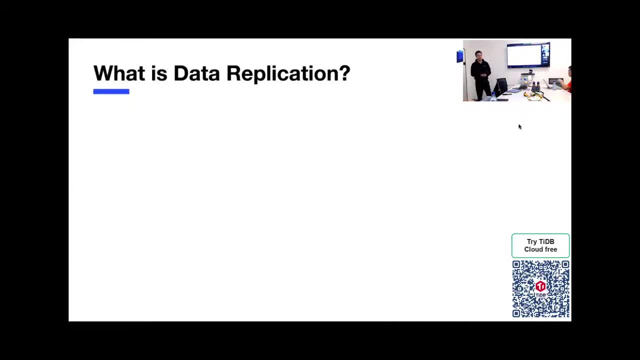 Okay, before we dive deep into the scenarios of data replication, I think two questions we need to answer. The first one is: what is data replication? Anyone want to have a try to answer this question? Anyone? Just copy of data? Okay, Yeah, Yes, data in database system changes dynamically when traffic red traffic. 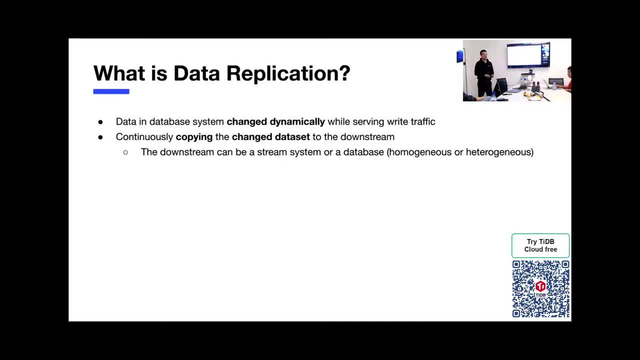 So the data replication is a process of continuously copying the data, the change, the data size from the upstream to the downstream. The downstream can be a system, a streaming system or a database system. Either way, Yeah, It is not a matter. The second question is: what is TidyC? Anyone want to try answer this question? 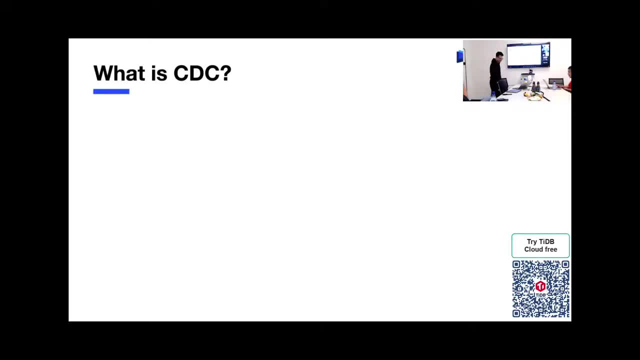 It's not the Centers for Disease Control. Actually, TidyC is a program. Is that the right answer? Change the data capture. Yeah, Okay, Right. Actually, it is just a program which is used to implement the data replication purpose. 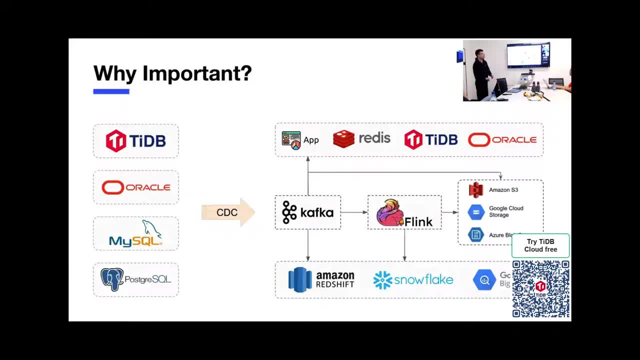 This picture, I want to highlight why CTC is so important. The left side is the rational database we are using and the right side is the other data processing components in our data stack. So CTC is the connector. Without CTC, our data stack is incomplete. 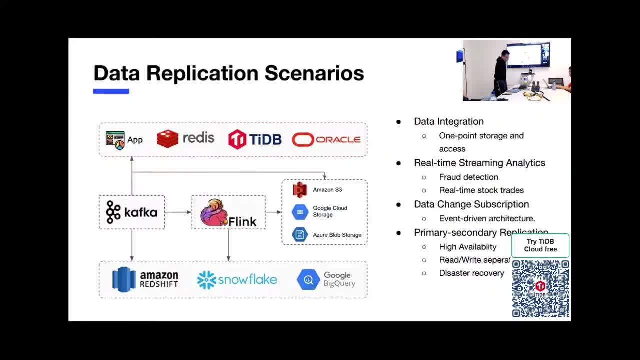 So CTC is very important. This picture is very, I think, complicated, So I classify into four scenarios. The first one is data integration. Data integration is the process of combining different sources into a single and unified view to make companies can enable the business instantaneous. 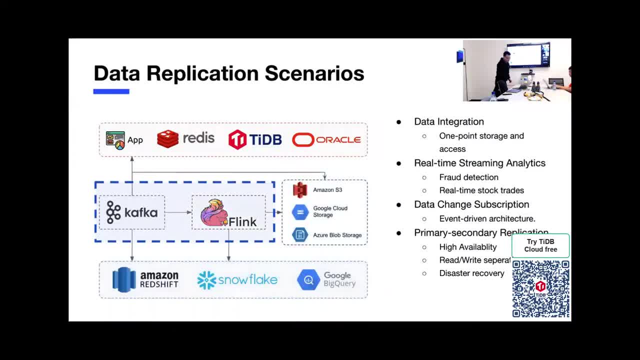 capability, And the second one is real-time streaming analytics. The first one- data integration- is just used for offline analysis, And the second one can make business more agile. The third, Oh, OK, The third one is, since the text and the square not match. 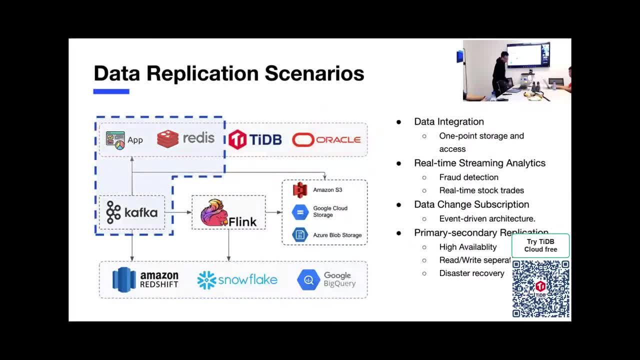 The second one is the change. this part Change data subscription which is used for implement the even driving architecture. We have a demo to demonstrate this. A lot of companies use microservices, Microservices architecture And the event drive Event drive architecture. use event to trigger the capital services to check different business logic. 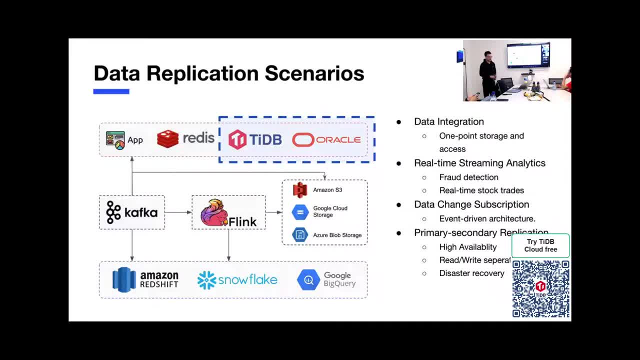 And the last one is primary signal replication. In the last decades a lot of companies use single instance database, So if they want to have high availability and scalability they must use primary signal replication architecture. In recent years a lot of distributed database system build and some high availability and scalability built in. 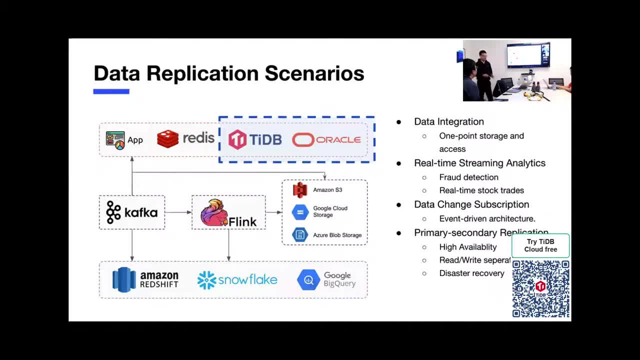 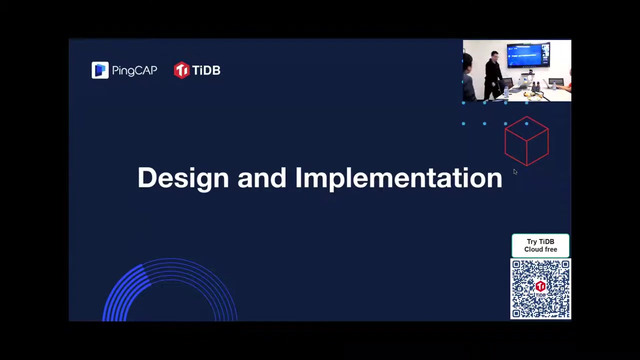 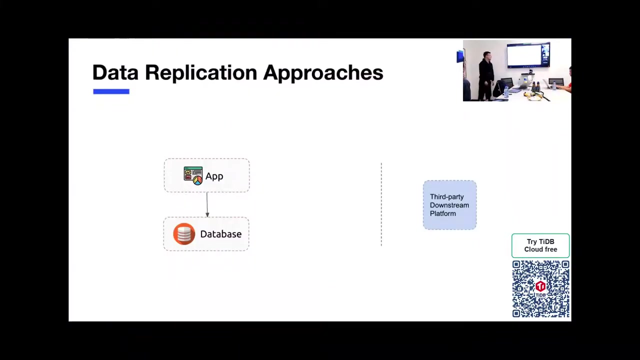 So this is a for distributed database system is used for disaster recovery scenario. A lot of financial companies must meet the compliance requirements, So they must use this, Use the primary signal, to meet such requirements. OK, Now we jump to the design and the implementation about the data replication. 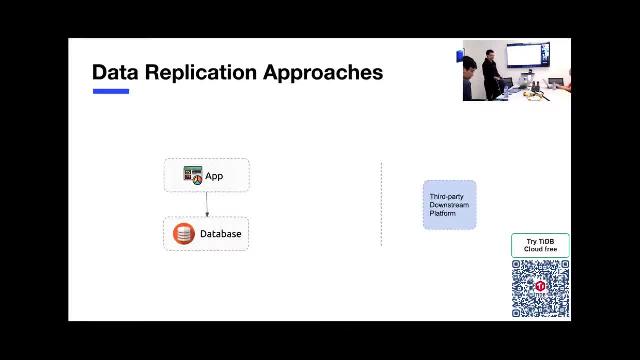 Before we dive into the implementation details, I have a simple question: How many approaches to implement the data replication? Anyone want to have a try to answer this question? Anyone? OK, I think you can implement it on the Any point of the data write path. 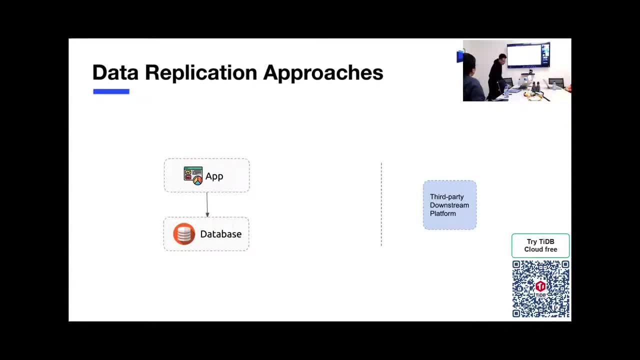 Yeah, Start from application. choose on layer database: Yes. Yes, First we can implement the data replication as a application because it's a data entry point. So before we implement the data replication, the application should be a data entry point. 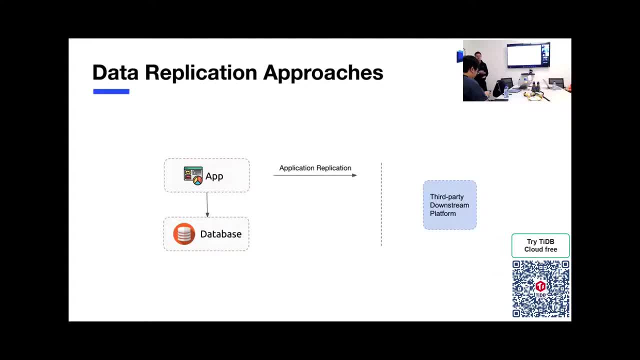 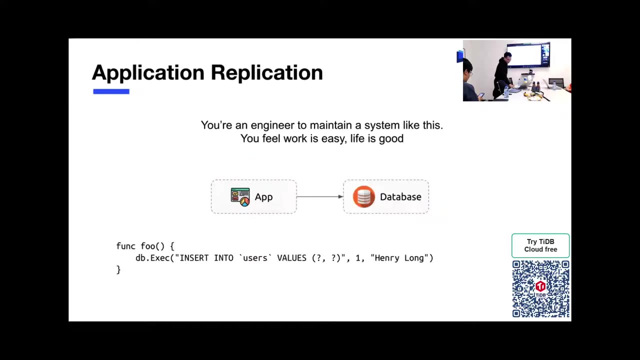 Right: write the data to the database system. we can write the data to other data systems as well. And the second: we can implement the replication inside the database. I will introduce the application layer replication first. If you are an engineer to maintain assistance like this, I think it's very easy because just application. 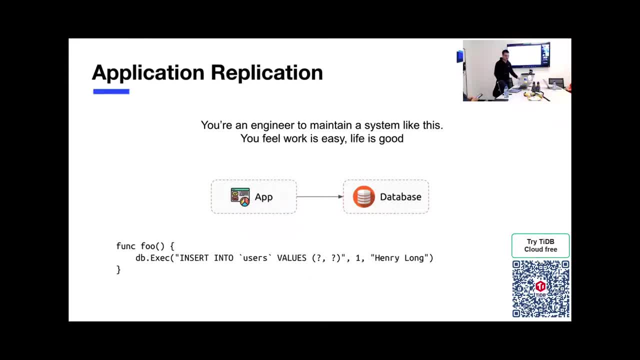 and the database. you just write some SQL and some code. One day. if you want to implement data integration- direct is one's choice- You just need to copy and paste your code again, again, again And you finish your task. And another day if you want to push the event to Kafka, add more. 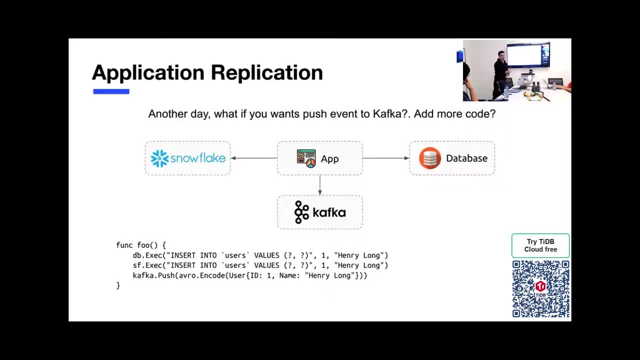 code since it works. We copy more codes and paste more codes, But as business evolution, it's difficult to add more and more downstream tags. So in this case, what do we do? For now, I think there are a lot of disadvantages of implementing data replication in application layer. So anyone 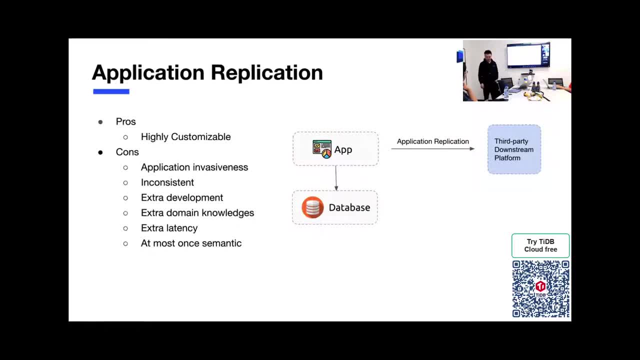 OK, We'll come back later. There are a lot of disadvantages to implement replication in application layer, For example. we must change our application and we can't keep consistent with different downstream systems And we have extra development and extra terminology. because you mustn't. 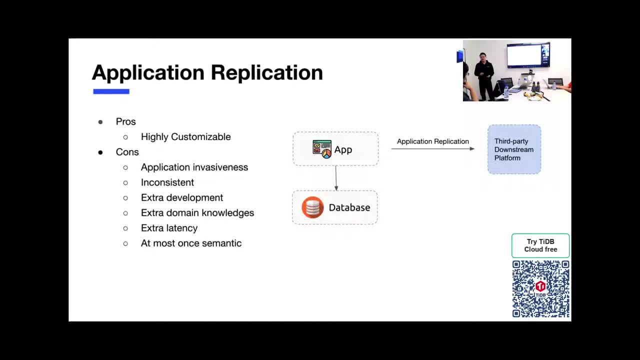 know the downstream system, You can talk with the system And we have extra latency because we We need to send the data to different systems. Even though we do such hard work, we just get the utmost once in every semester. I think there is no cost effective In this case. what will you do? 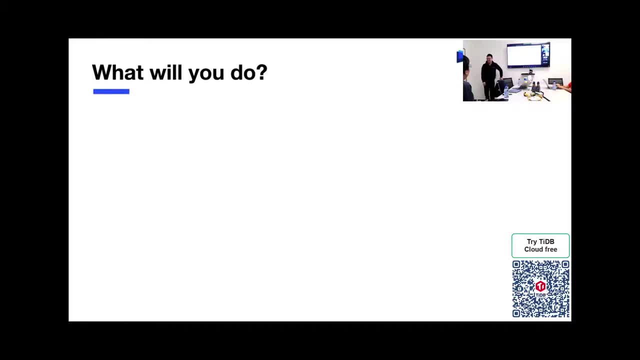 In this case, I will choose the replication between database, and I will use BIMBOT And then write a BIMBOT to Kafka and then subscribe to BIMBOT. What if the database doesn't have a data replication capability? I will pick another one. 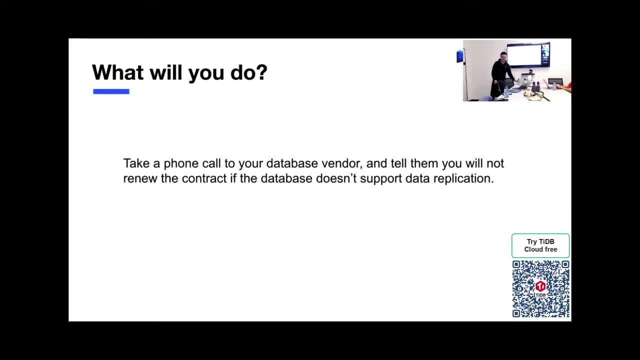 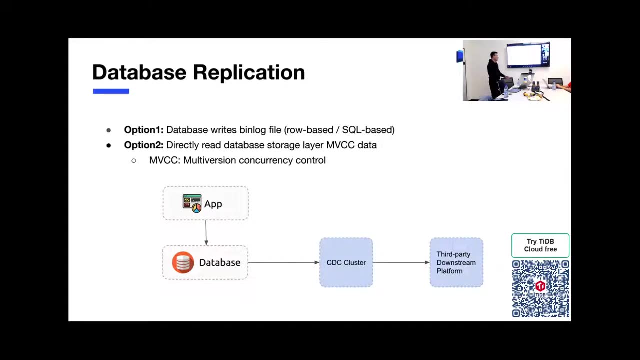 A simple suggestion: take a phone call to your database vendor and tell them you will have to review the contract if the database doesn't support the replication. So the database vendor will try hard to implement this feature. Actually, there are two options to implement the data replication. 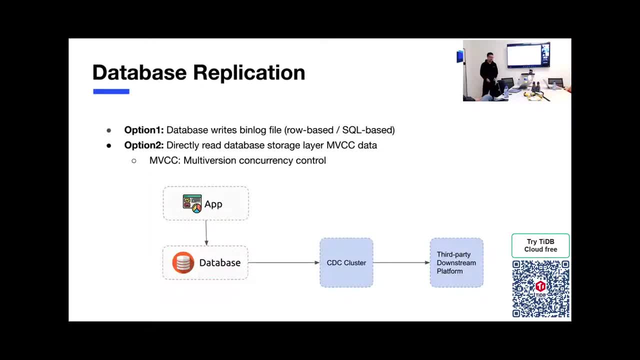 in database inside. The first one is write a BIMBOT file. you mentioned before Write a BIMBOT file. we have two formats: a row-based format and a single-base-based format. For the option one, there is still some disadvantages because it has a write path which we need to write. 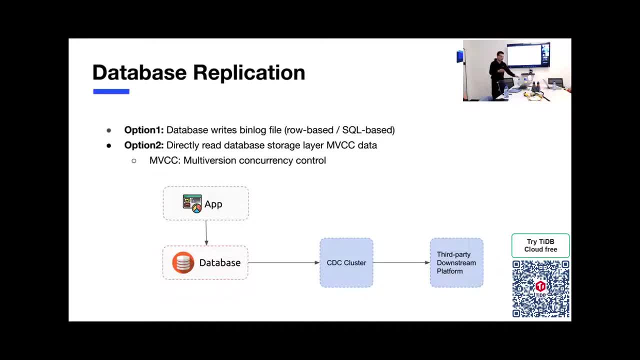 Even though we write the data to BIMBOT file, there is still extra latency. The option two: directly write database storage near MVC data. MVC data is multi-version, concurrent and continuous. I will not going to introduce the MVC detail. I think a lot of materials on the public resources. 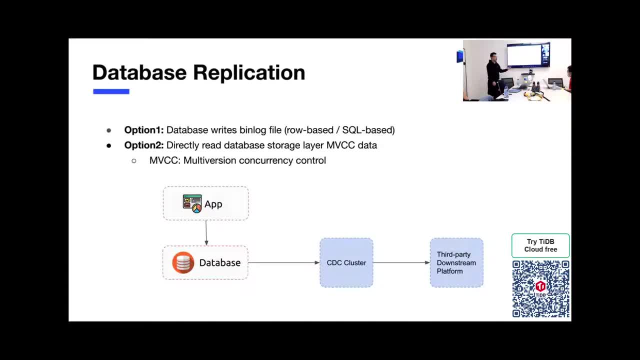 You just need to read the MVC data from the storage layer and retrieve the changed data side. There are a lot of advantages of implementing MVC data. There are a lot of advantages of implementing MVC data. There are a lot of advantages of implementing MVC data. 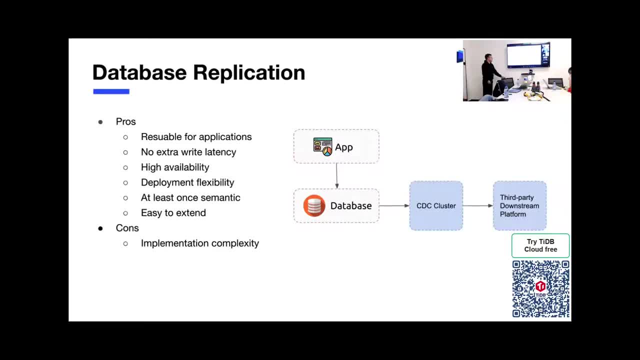 A added plus advantage is carafecting UTK and database side, because we can resolve carpeting for every application and low extra latency. The degree of availability Deployment is very flexible because it's an external component and the we we can guarantee at least once download a deep binary format. 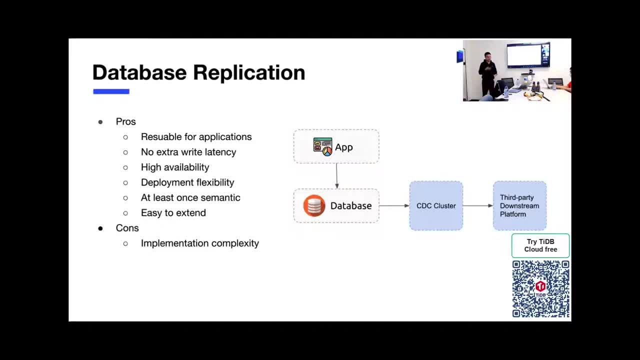 and easily toprove containerigt while writing memory. complex IPs extend because we extend in external component and we can upgrade the component to individual. The only one disadvantage is implement. such a system is very complicated because we must also know the implementation detail of storage layer, For example the transaction. 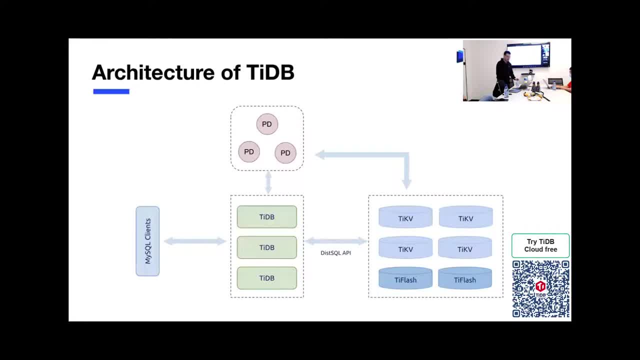 in the MCC. I will introduce the details of our implementing the TIDCDC. This is a high-level architecture of TIDV. This is PD cluster. PD cluster is used to store the metadata of the TIDV cluster. You can trace the brain of the whole cluster. 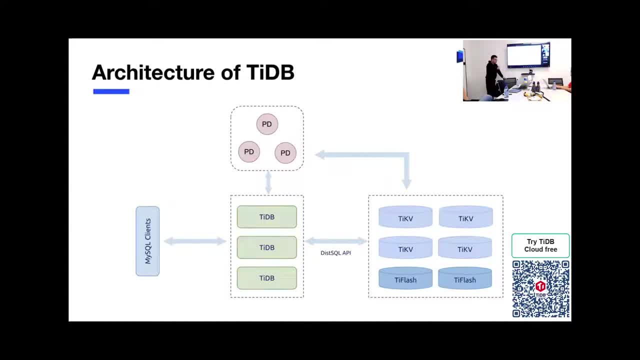 The TIDCDC is a SQL layer. It is a compute load. All the application talk with TIDV and TIDV talk with the storage layer. Our storage layer contains two storage engines: The TIDV is a row-based storage engine and the TIPLASH is a. 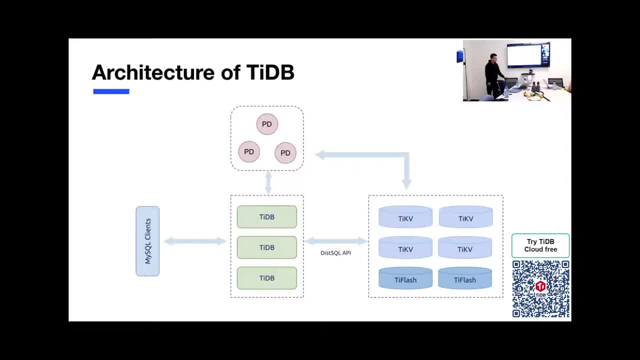 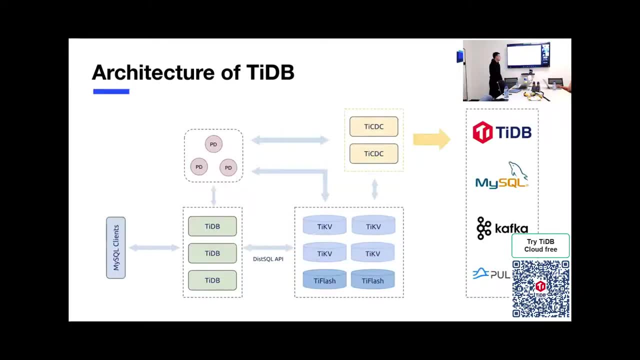 culinary storage engine for analytics. That's all you need to for subsequent slides On this page I put the TIDCDC into the TIDV architecture. TIDCDC talk with PD to track the metadata of the storage engine and then read the change, the data from the storage engine. 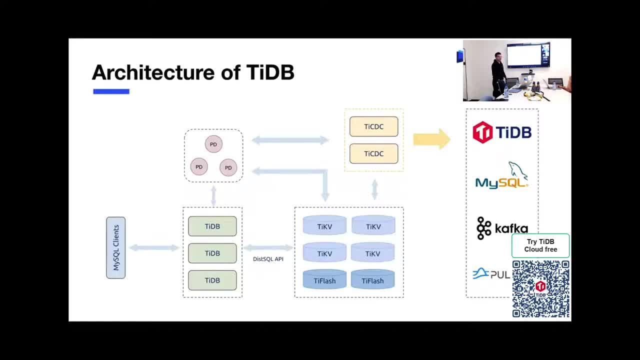 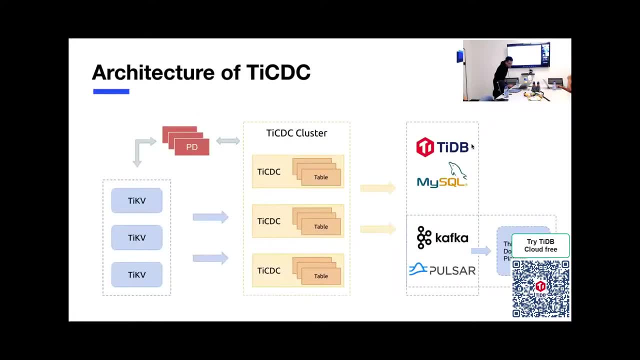 What is PD short for Placement driver? Placement driver. yes, Let me see. This picture contains some internal details of TIDCDC. TIDCDC is a highly available system. TIDCDC cluster contains a lot of TIDCDC loads. Every TIDCDC load serves a bunch of tables. 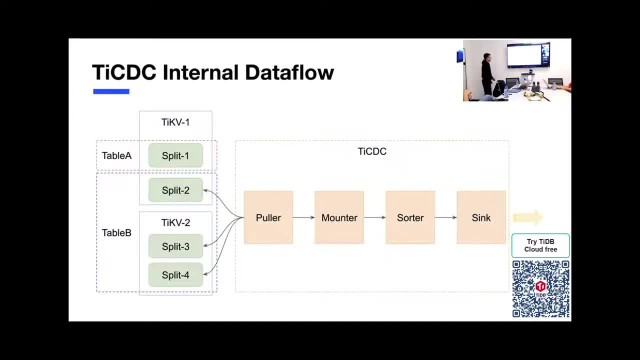 This picture shows the TIDCDC internal workflow. Our table consists of a group of splits. The splits can be placed in different TypeKV loads In the TypeCDC site. we split the whole data pipeline into four modules. The first one is Pooner. 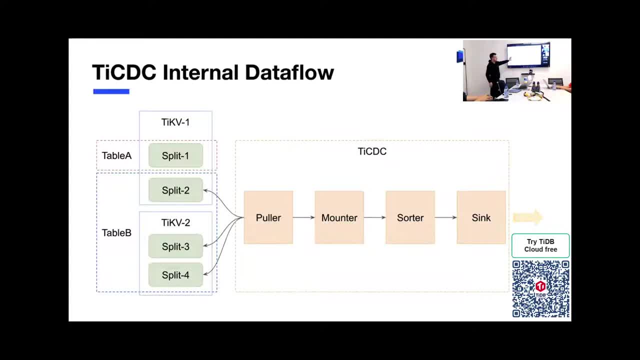 The Pooner is used to pull the data set from the TypeKV. The Pooner pulls data using k-value. The monitor is used to convert the k-value data into rational data. The sorter sorts the data ordered by the transaction ID. 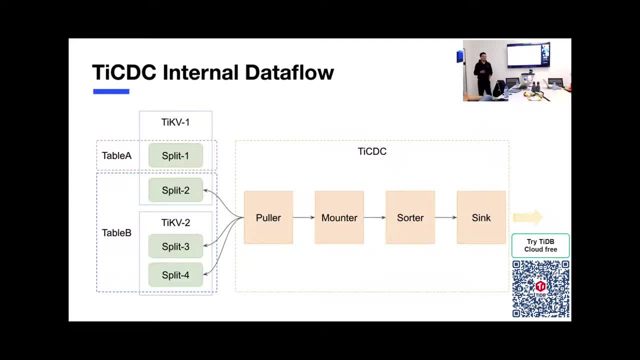 The sink adapts to the downstream protocol. That's the data. That's the data to downstream. What is called a monitor? Actually, I don't know, It's a decoder. I guess A decoder is a much simpler name to talk about. 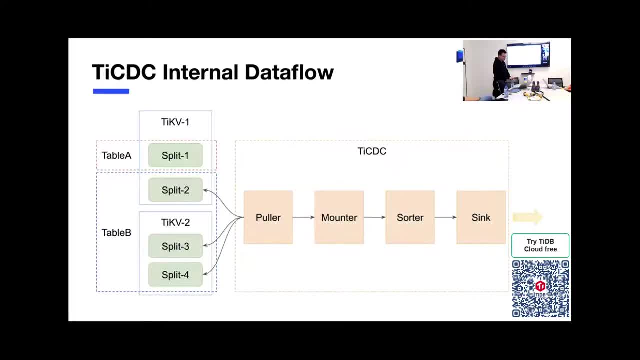 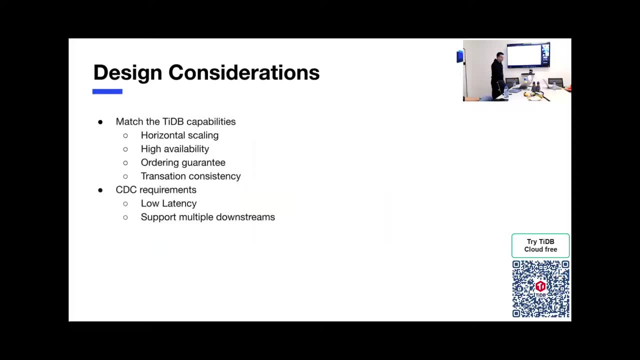 So within the database, all the changes are in order delivered. I will mention that in the slides. There are six key points when designing the system. The first four is to match the TypeKV capabilities, Because TypeKV is a horizontal, high-availability, transactional, scalable database. 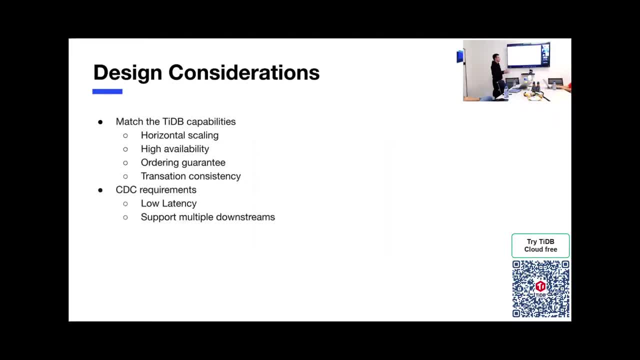 So the TypeCDC must match the capabilities for the horizontal scanning and high-availability ordering. guarantee and transaction consistency. The other two requirements is from CDC. CDC is used to synchronize the data set to the downstream. They must provide very low latency for the synchronized scenario. 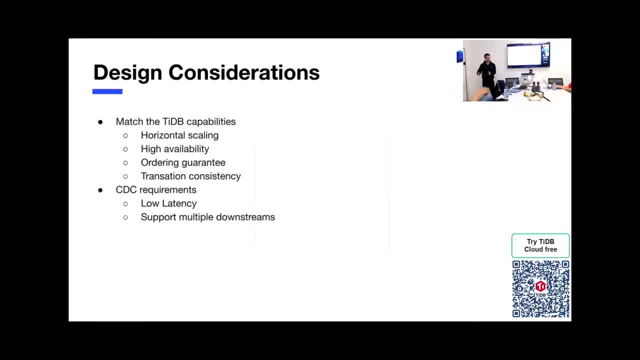 Because the CDC is a connector of TypeDB and the TypeDB system, so we must support multiple downstreams. Does that make sense? Okay, So the first one is horizontal scanning. Any system want to have the horizontal scanning capability must have to solve two key points, I think. 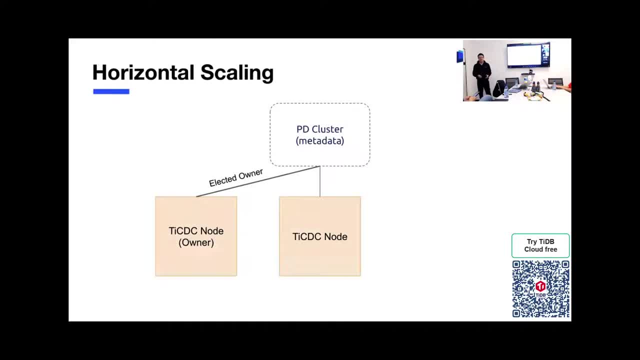 The first one is discover the newly added load And the second is balance the workload And the third one is to manage the cluster. So this example: we have two load in the TypeCC cluster And the one TypeCC node will come in to be later and success. 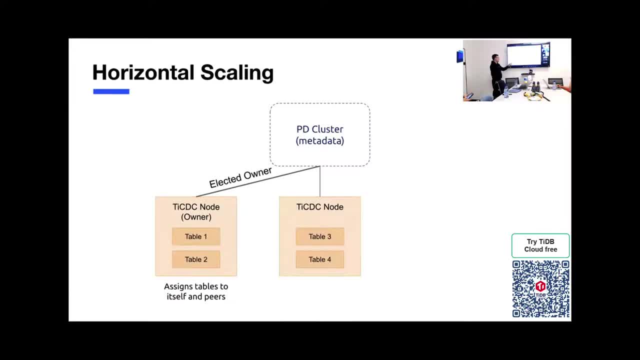 This is the owner, And then the owner is responsible for assigning data to itself and the peers, In this case the two nodes. In this case we have four tables And each TypeCC node serves two tables. When we add a new TypeCC node, in this case the owner will discover the new load added to the cluster and try to migrate some workload to the newly added load. 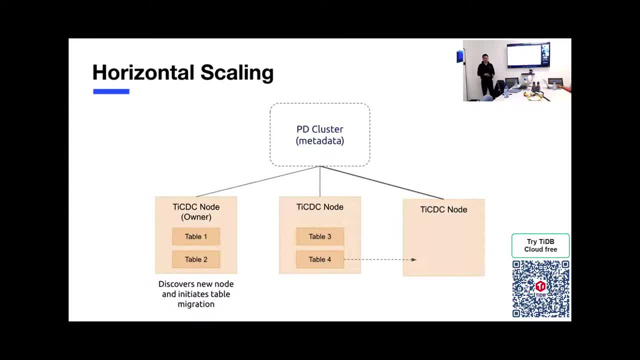 How to discover the new load. The owner will watch a specified key And if new load register, they will put a new key to the key space And the owner will discover new load added in the cluster. So it's based on the table or it's based on the sorted key string. 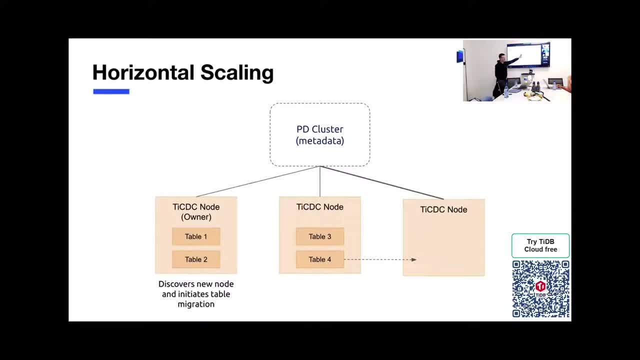 Based on the PD cluster. I think she's asking that because it's table-based. Okay, Is balancing a problem? I think change is based on table. Yes, for now it's based on table. I see. So if a table gets too big, then 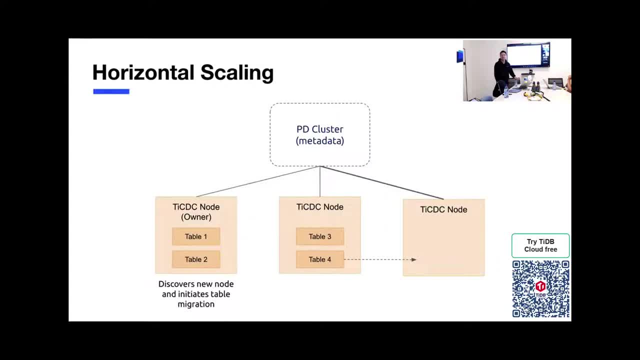 Yes, Yes, So it evolves like data movement from one cluster, sorry, from one node to another. Or does it just go in this table, right? The data stored on TypeCC, TypeCV. So when the owner tries to migrate a workload from this node to this node, just the cooler. 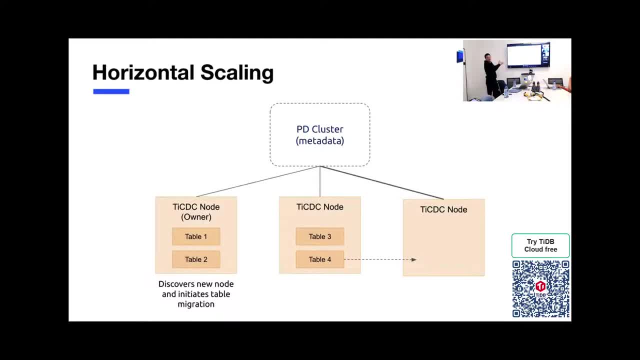 runs in the CC node And the data is still on the TypeCV storage engine, So we can conclude that this is a state list. Yes, Yes, It will be mentioned in the subsequent slides. So you mentioned it's in order. Does in order mean it's in order within a table where it's in order globally within? 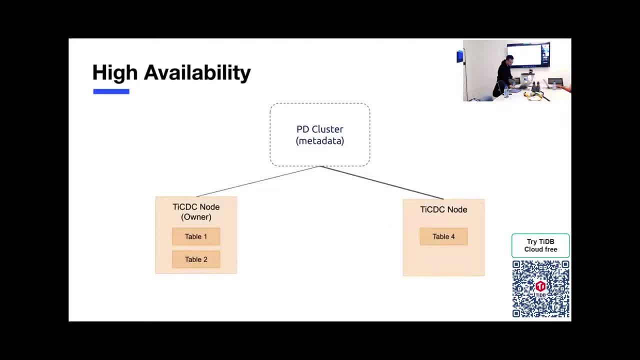 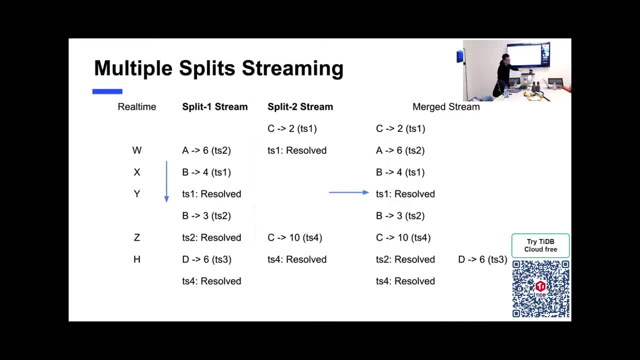 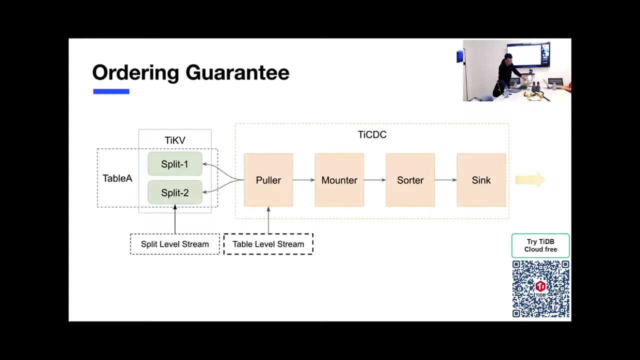 a database where it's in order within a node. This part, Actually in the different stage of the data pipeline, we provide different level of order. Okay, Yes, The next subtopic is have ability. There are still two key points. 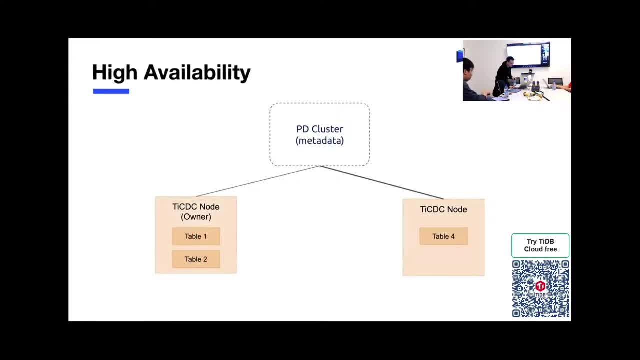 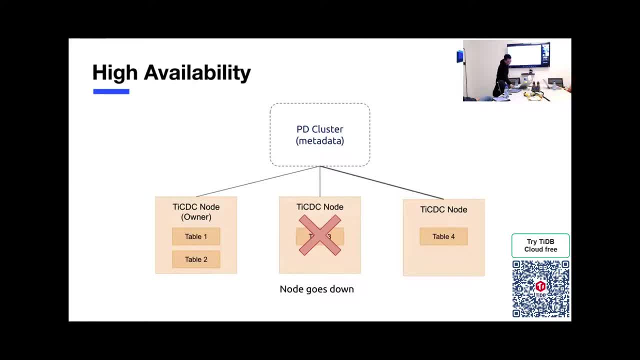 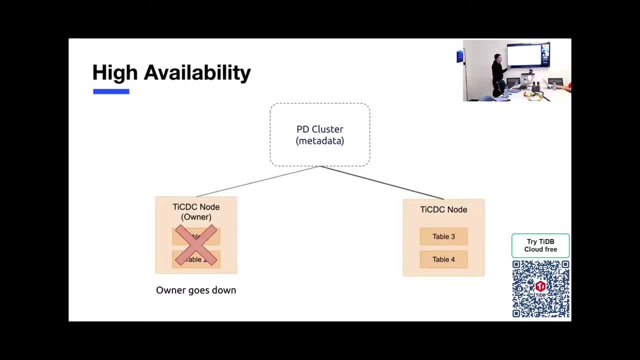 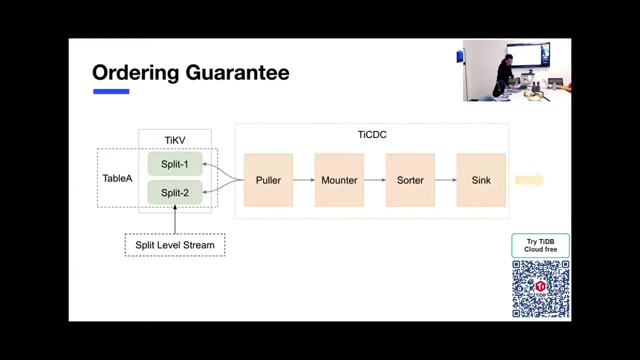 What if owner goes down? The surviving load will try to campaign to be the owner, and this does the owner lantern the workload to the surviving nodes. Okay, This is the next subtopical. It's the ordering guarantee, Because every shot outputs a stream individually. So 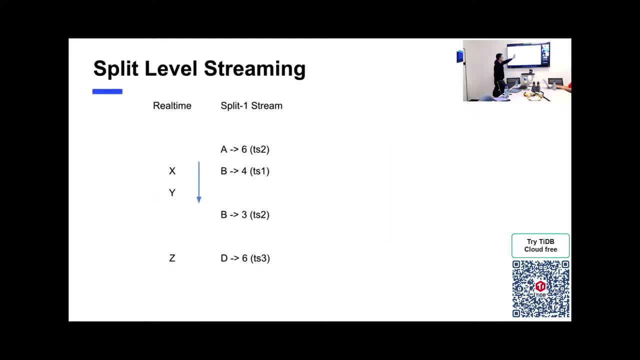 In this example, split stream. In this split we have three case and data changed into transaction. Every time stamp represents transaction We use resulted TS to indicate the watermark of the stream. The watermark is: is a minimal implied commit TS. Commit TS actually is the timestamp of a transaction committed. 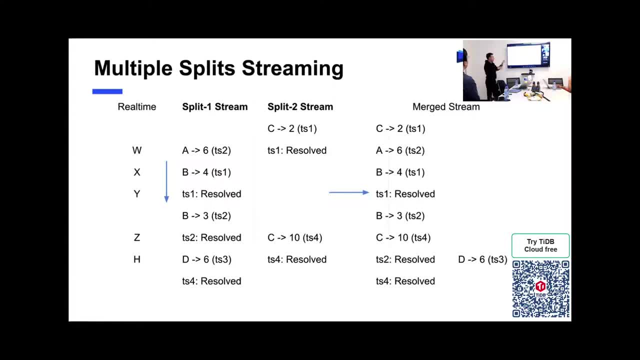 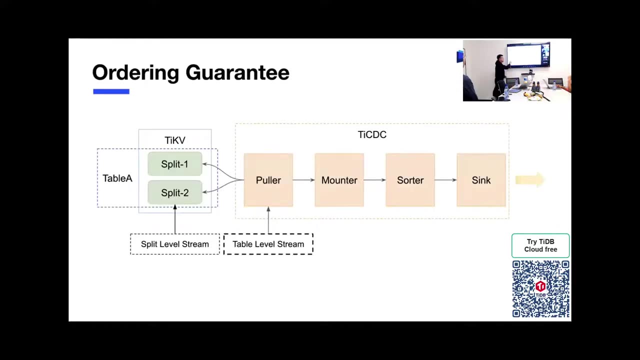 For two split scenarios. the pruner will merge the two split streams into a merge stream to keep them in order for table level. So this split output or split level stream, it's ordered just in the split. The pruner merged multiple split and output or table level. 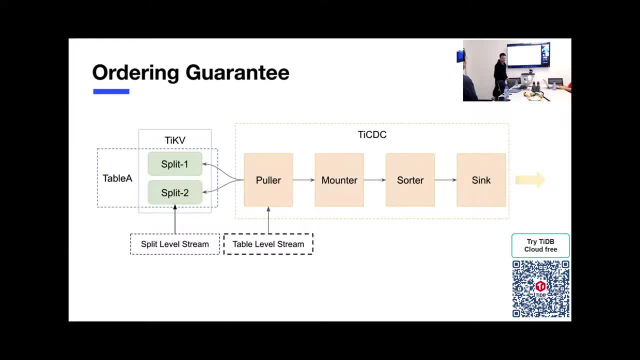 order stream. Sorry, what's the key for the order Key? Yeah, yeah, You order by column. Order by transaction Transaction ID. In this case, because every transaction may be a cross-table transaction, the pruner outputs just one table. 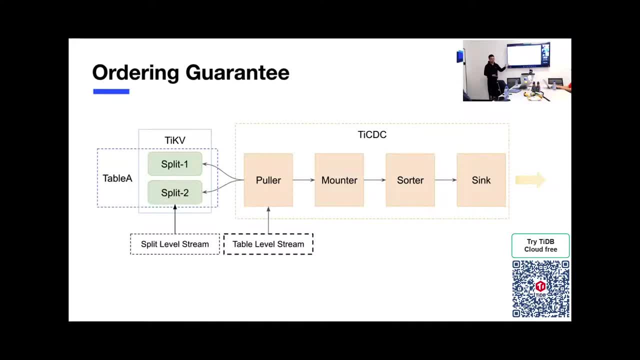 So ordered by the transaction TS. Yes, ordered by the transaction TS. Okay, Pardon me, who assigns these TIs? PD cluster. Yeah, the PD cluster has a TSO service to relocate the TS. How do you decide? or how does the PD decide? you know where is the time to assign, et cetera. 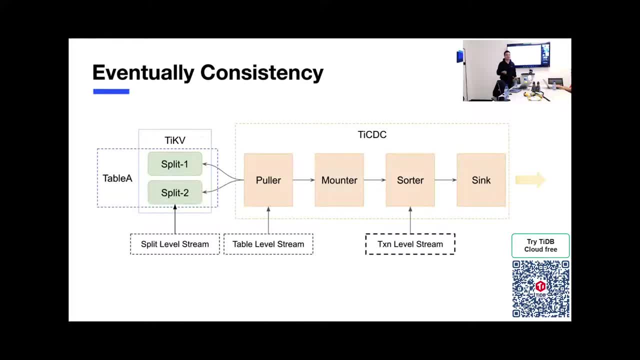 It's a more increased number, I think just. I know that. It's just like when you put it like, for example, I have a, I have a commitment, I have a commitment right. I have a transaction and I have some statement right. I say: we have row base, okay, So you have some statement. 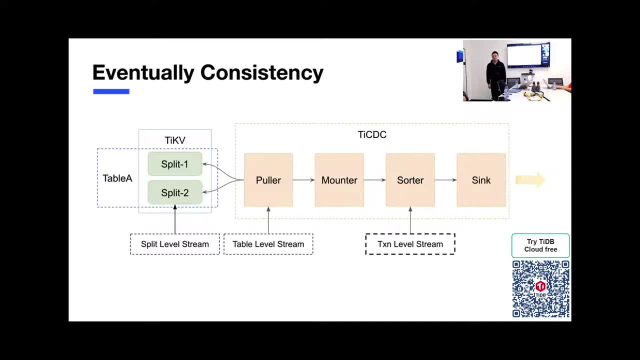 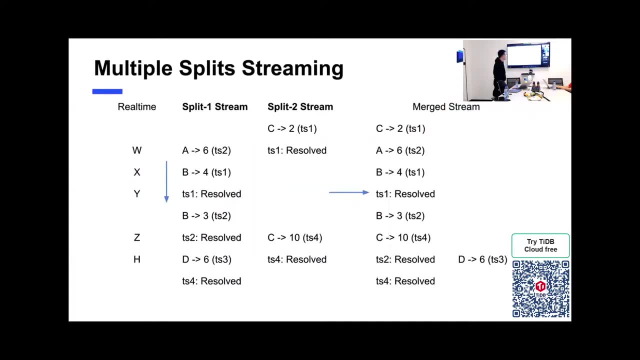 sorry, SQL base. okay, You have a statement. So how like could you please go back to the? you know, like previous, like yes, Which one? Yeah, so when you do the merge stream, right, Okay, 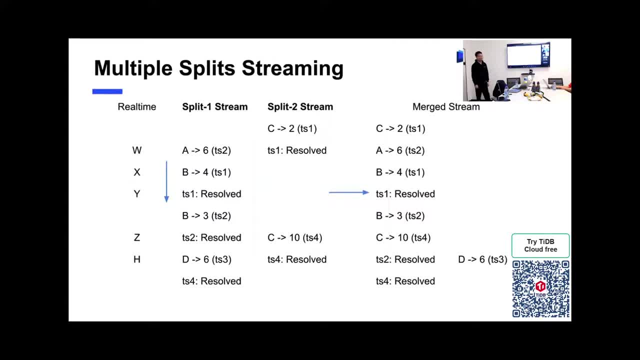 When, how? let's say like say N and B, how do you decide like this, say A, B, and you just say like TS1 resolve, which means okay, I'm sequenced. the R's are already settled. 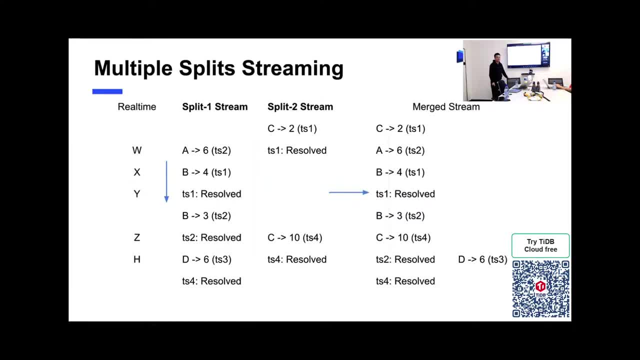 So what's the what's the, what's the criteria of? you know, sequencing these three events, you would say like or three, some module would: how is the sequence like this? or whether this order should be reversed or not. 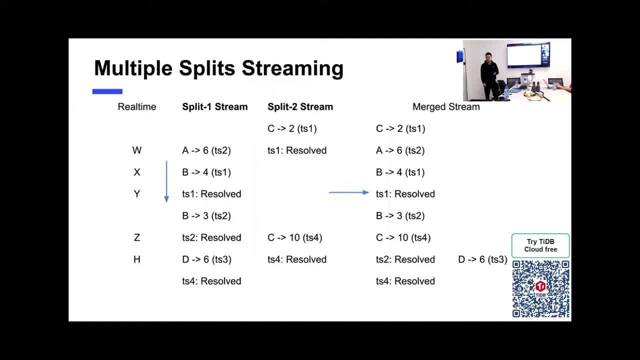 I'm trying to based on the value of the timestamp. Okay, So the timestamp. if timestamp is larger, then it should be order in the back. So every statement you will assign: I'm sorry, TS No, Transaction, Transaction: yes. 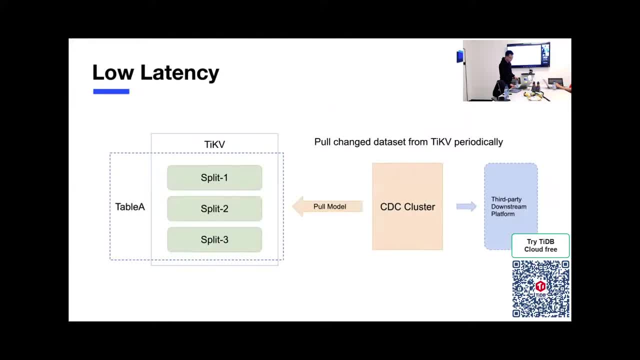 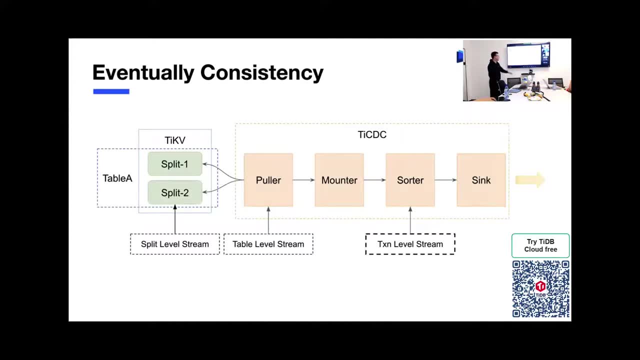 So every time you commit then it will allocate a timestamp from PD. Okay, And every key will have that timestamp, All right? Yeah, This order is because the footer just outputs a table level string. they bat a transaction, maybe a cross table transaction. 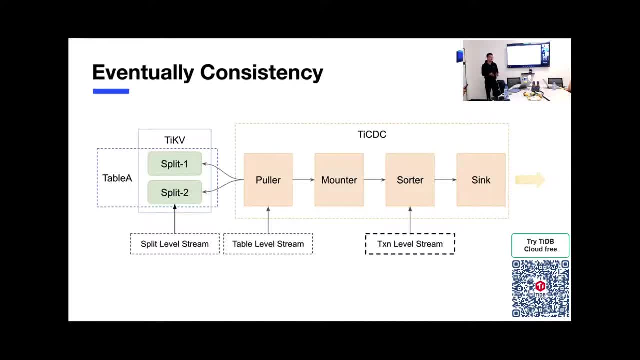 So we we must have kept the kept all tables in transaction in the same piece. So the, the order will control the, the. it will sort all the merge stings and replace the transaction to the session downstream and control the watermark of the stream. I'm sorry, I lost my mind. 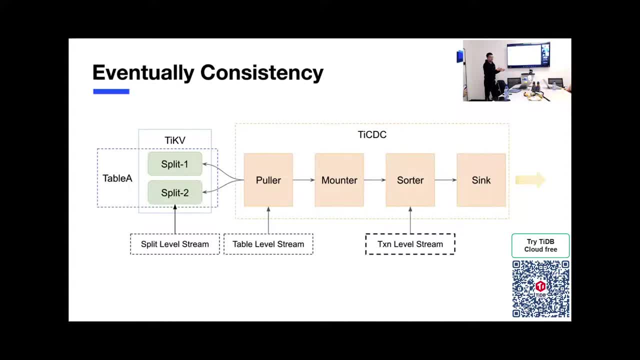 I'll say the sorter will sort all the merged streams and keep all merged streams into the same place to replay the data into the downstream system. Does that make sense? So you have a cache of the table stream before it's being replayed? Yes, we have a cache Because we must make sure that all the data 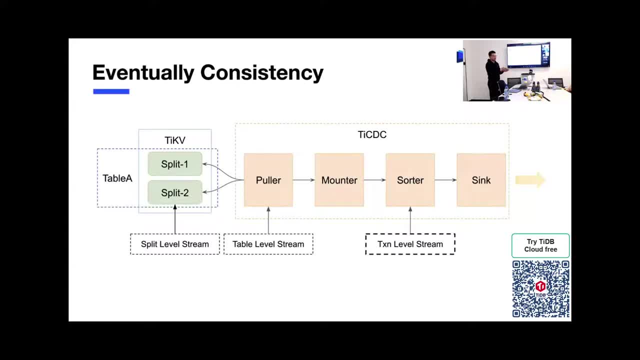 read to the downstream. before this transaction We will clean the cache to ensure the consistent inventory. So how can you advance your watermark? If the transaction submits to the downstream, I will advance the, But the stream they are not still. I mean the stream arrives at a different pace. 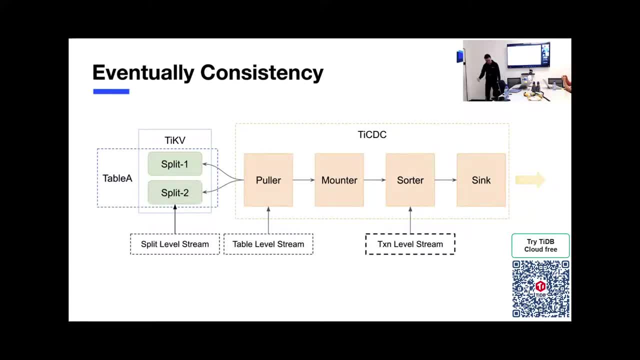 What if one stream arrives late? Have a cache. They have the result timestamp to determine, I think before this. the result type means that if you see this result here, which means that you have seen all the events happened before this result here, So you can. 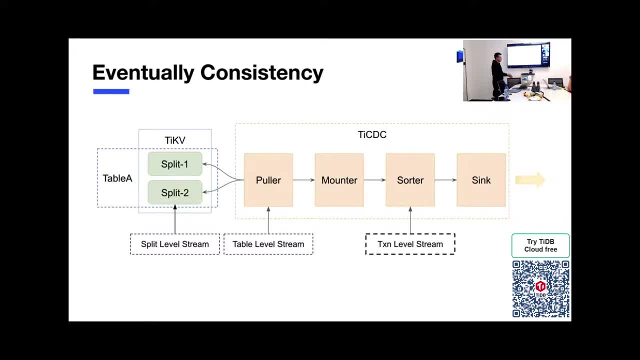 What transaction before this result here has been: Yeah. the result here is critical here to determine when to dispose of those changes to downstream. Oh, this is kind of Yeah. So even though you have a lot of, You know, the sort is on one basically. 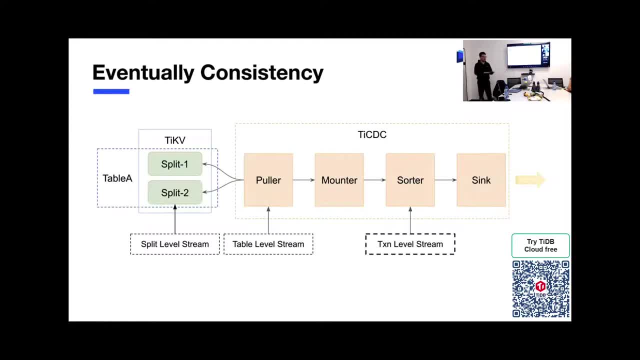 Oh, no, no. no, Then we are exchanging the TS peer-to-peer, and only if all data before this TS submit to downstream and the TS will be advanced. The peer-to-peer exchanges the timestamp information, So there's any out from the downstream. 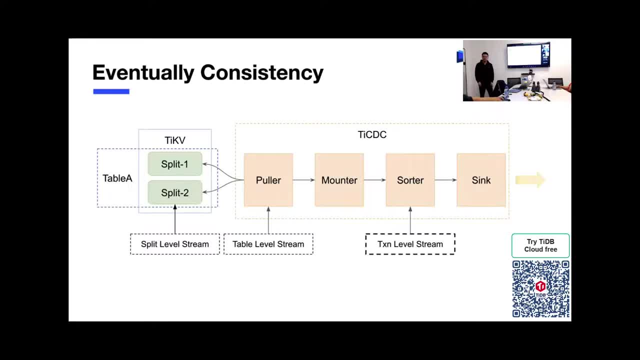 Or just like I send it off and I'm done, And just a little on slide, Yeah. So what's the mark of margin and of like a TS? How can I advance it? I think I'll go back to how the result TS is completed, right? 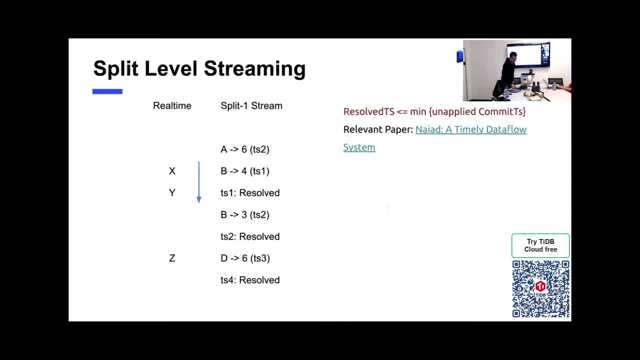 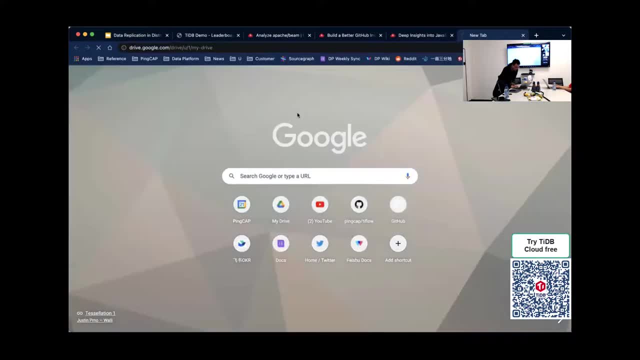 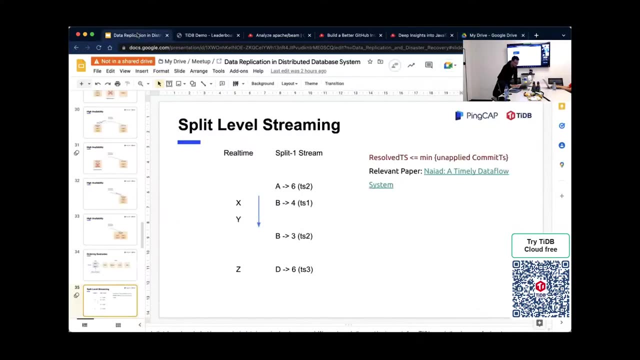 It's a lower bound of Actually. result: TS has a very complicated, Or what is it? It has a very complicated, Oh, what is it? It's a lower bound of a TS. Yeah, So basically, as far as we write, transactions are ongoing, committing right. 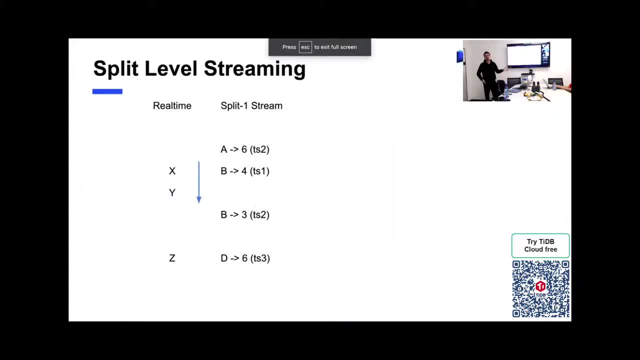 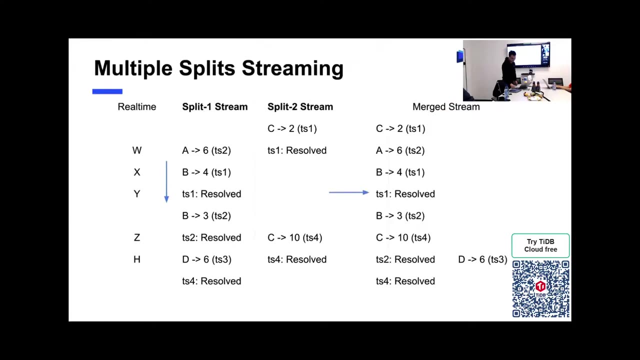 If you're interested in this class, I can show you a document about how to calculate the result TS. It's very Complex, Yeah, but basically the idea of committing transactions higher and higher timestamp determines the downstream, how you can push those changes to. 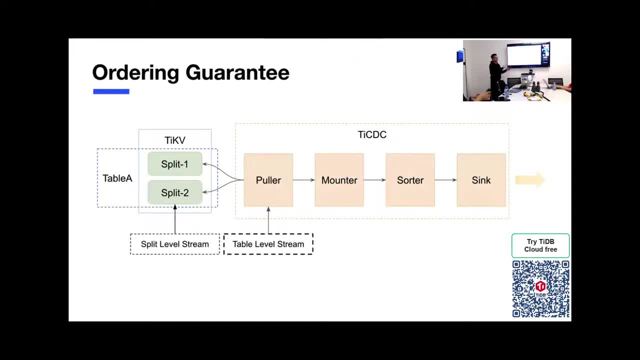 Because it's. The cluster is a dynamic system. All the speeds in the TICV are scheduled every second And some TS node maybe goes down. So it's a dynamic system. We must To determine a watermark in the dynamic system. 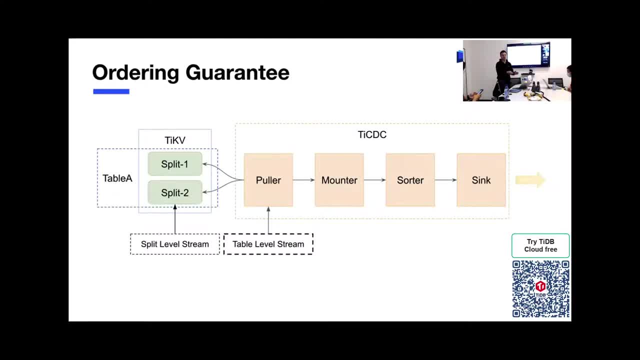 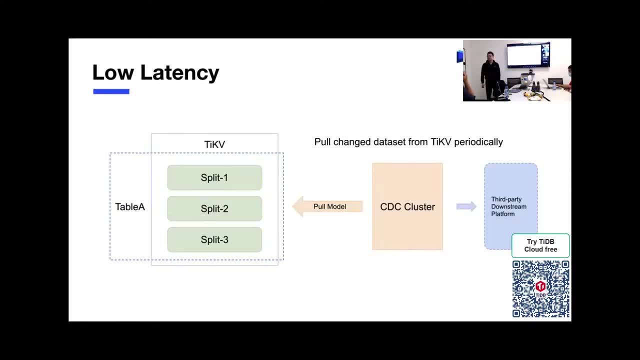 So we have a very complicated algorithm for this. Also, I think the key thing here is that because a transaction can And once you make those changes, because when you commit, this commit happens in asynchronous fashion, which means that those changes A transaction may commit first, but then you refuse, changes may arrive later. 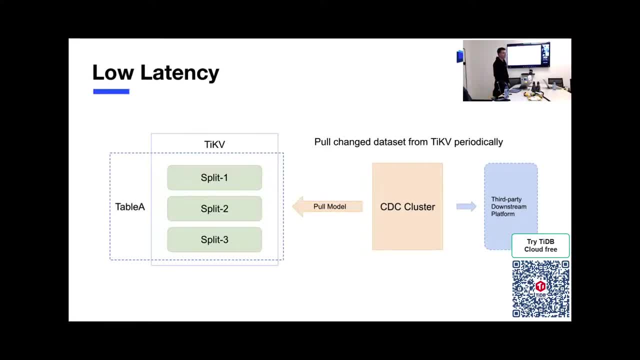 That's why you have to have some sort of buffer and wait for the result timestamp before you can safely make sure that It's an old transaction of an earlier timestamp And then sometimes Otherwise you'll wire it. So it's like a transaction guarantees. 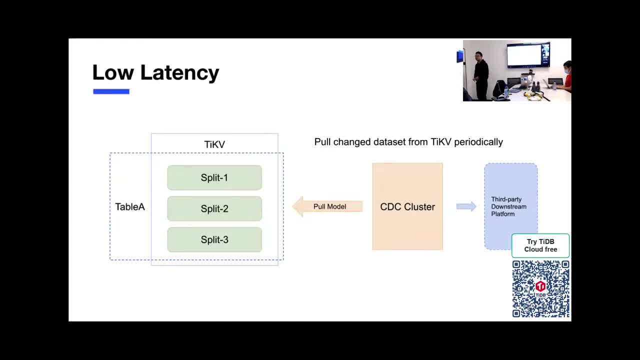 Yeah, that's basically the idea. Then you don't know the order between different nodes And you need to, in a central place, reorder those. We have two CDC nodes and two streams. This stream is Table A. This is a board. 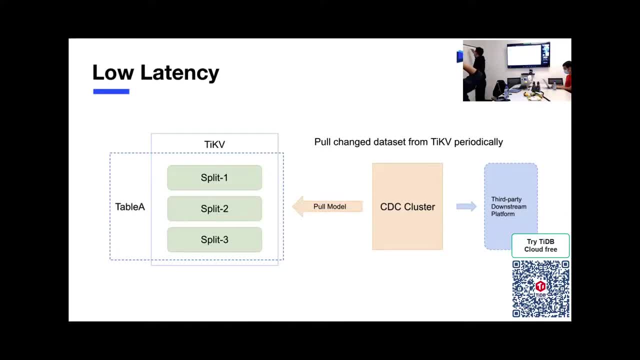 The transaction. How about we discuss this later, Because I think the people online cannot see the whiteboard. Okay, okay, Yeah. The next subtopical is low latency. We have two programming models to retrieve the changes that they set. The first one is ProModel. 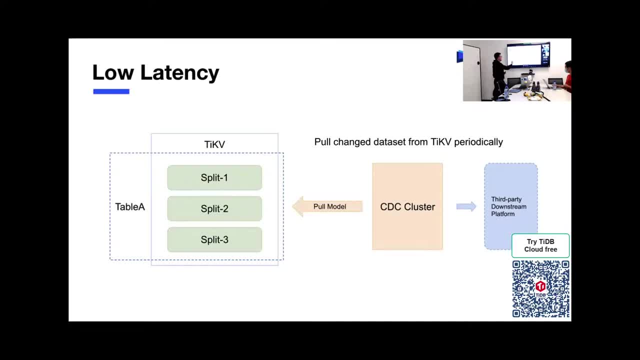 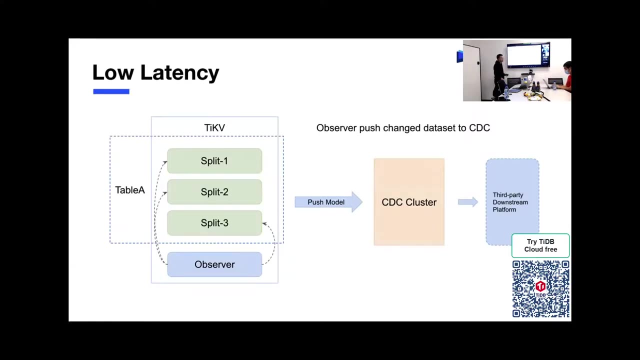 We can pull all the changes that they set from TechKV. Practically this is like the Kafka consumer And we have another way is the push model. We can implement a module in TechKV and to observe the data change and push the data. 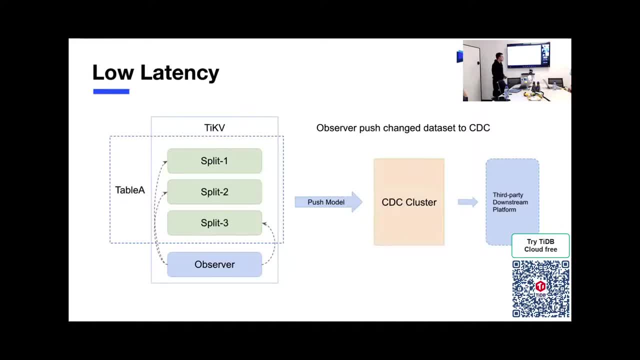 to the test in time. We combine the two program model to achieve low latency. They use the ProModel to trigger incremental scan, For example, when I'll say: When the load was dropped there wasn't a pull request to the TechKV. 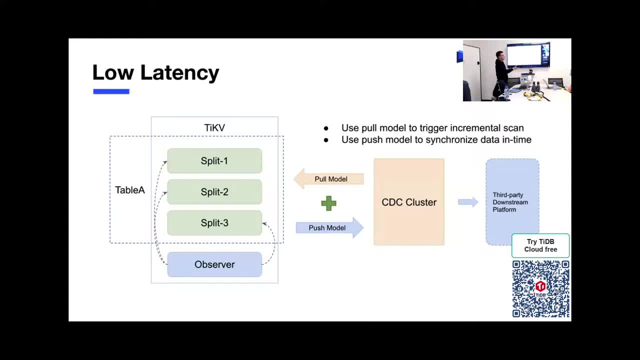 And TechKV will scan the chain data and send it to the node And after all the chain data is sent to the cluster, All the fresh data changed in the TechKV will be used. push model: Push the latest data to the CC load. 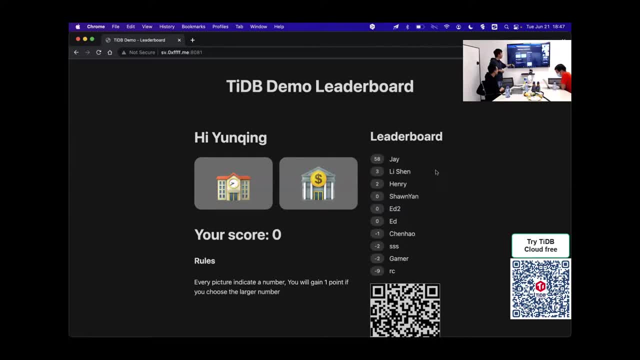 If you win one point, if you choose the wrong one, you will lose one point, And for each round the change of score will reflect to the leadboard immediately. So this is a dummy game. It's to show the capability of HiCDC. 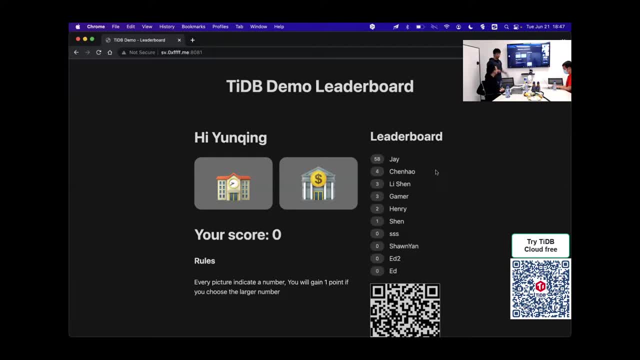 So, yeah, you can join the game and click on the image. Have a try, maybe. OK. OK, It's Yunqing. Yeah, You can see. I was wondering. Yeah, Why is it me? You can see, during the play you're playing, the leadboard keeps refreshing. 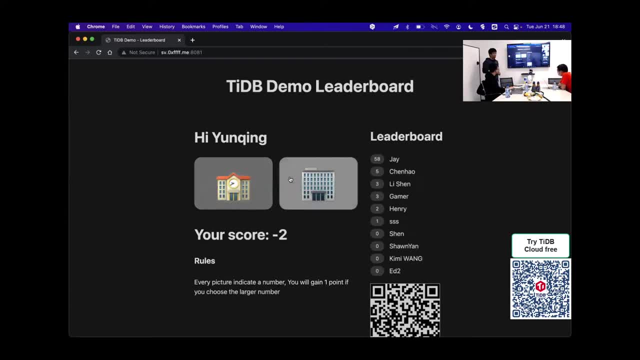 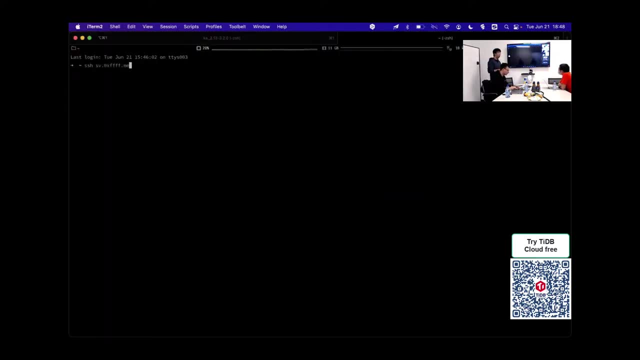 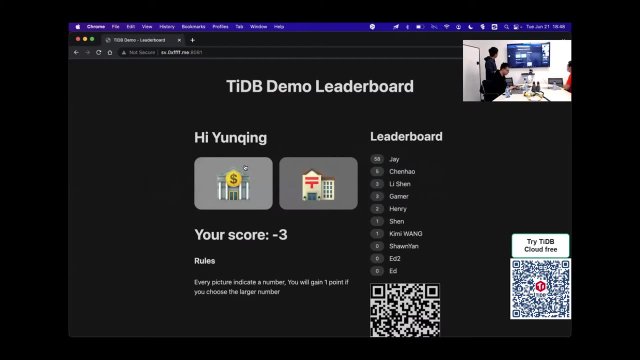 OK, So this is a simple game And it's just to show that with HiCDC, we can replicate data from the database to the downstream in quite a short time. And yeah, For the next time, Henry Miss Bloom will kill HiCDC. 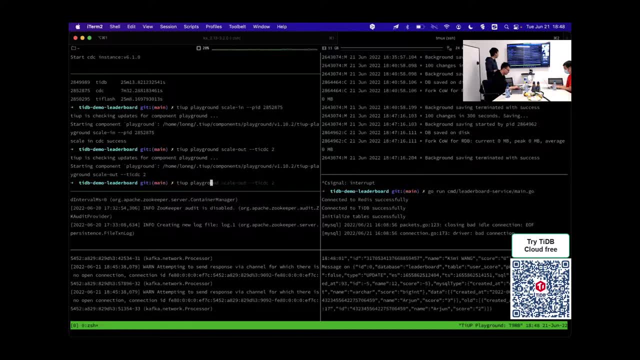 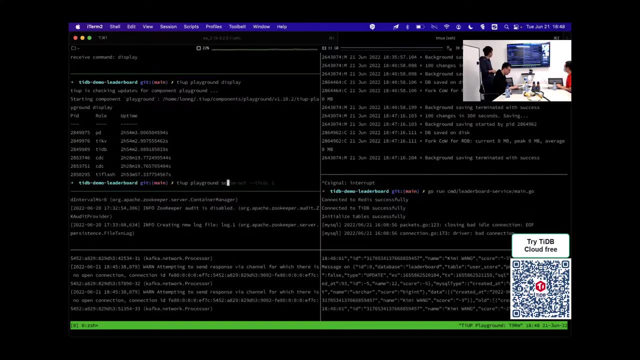 Will kill one. Kill the TypeCDC nodes to show the high availability. Yeah, Yeah, I will. Yeah, OK, All, Yeah, Fair. please Can you increase the font size? OK, OK, OK, Yeah, Here. 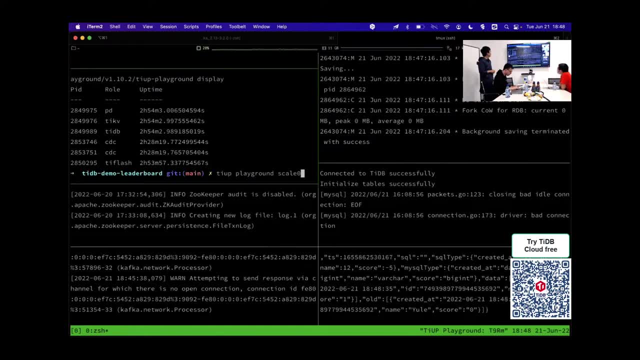 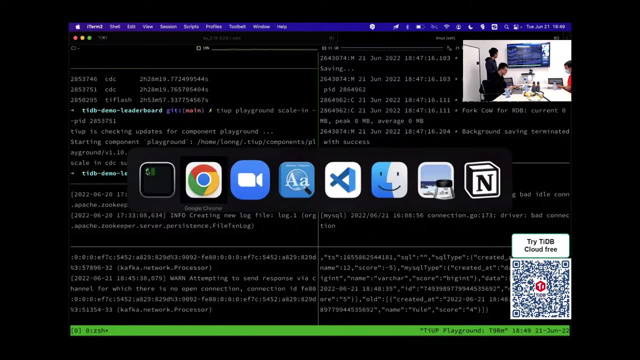 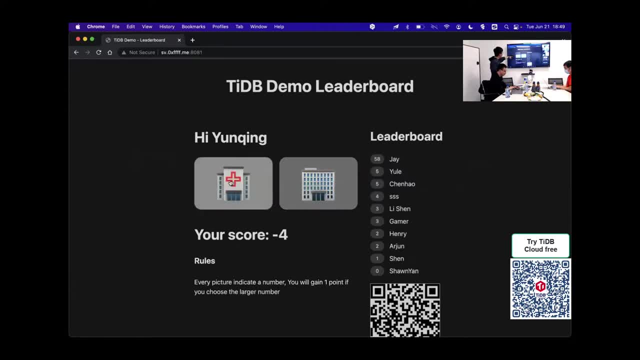 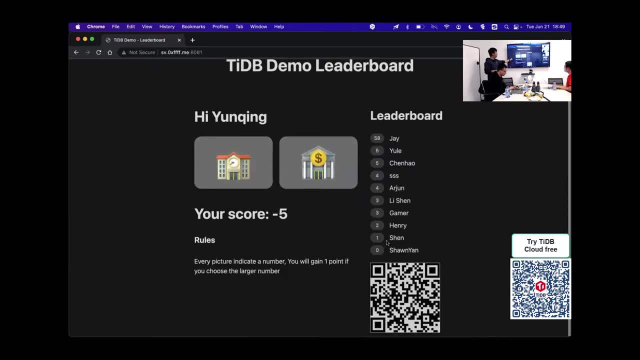 The number is still jumping. Yeah, yeah, Yeah. So you can click on the picture to see. You can see, Even there is one TypeC instance called The system can steal synchronized data to the downstream, So that demonstrates high availability. 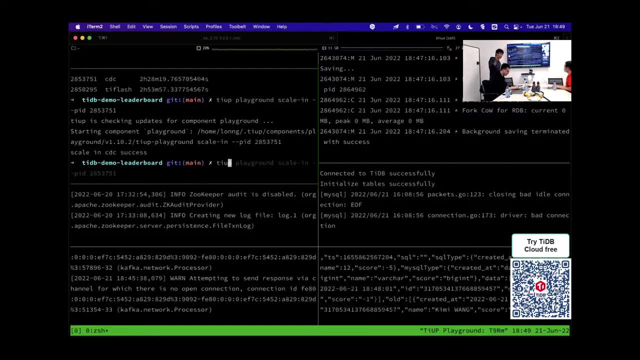 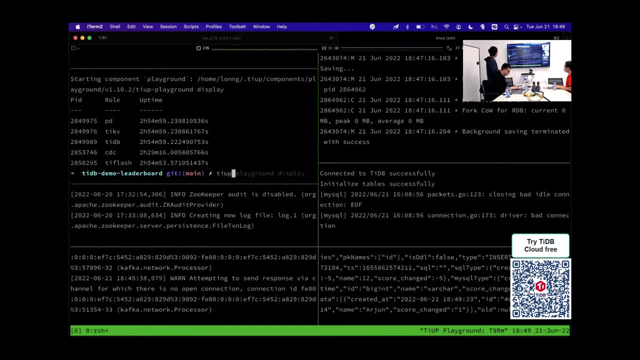 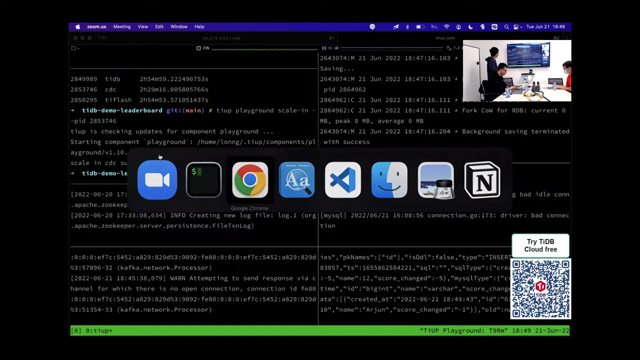 Maybe you can kill another one. I think there's only two instance out there. Yes, OK, Okay, there's only one instance. pass the instance there. Okay, Let's go back to the to the browser. Yeah, Let's try to click on the on the picture.